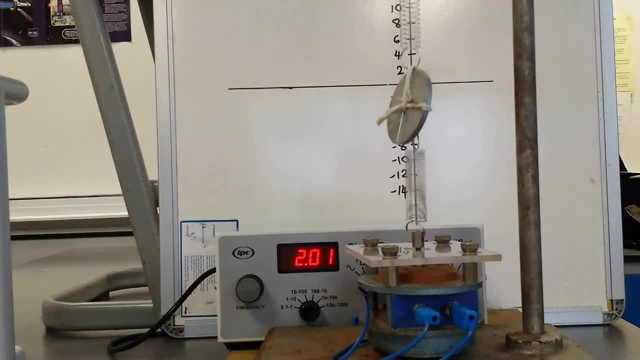 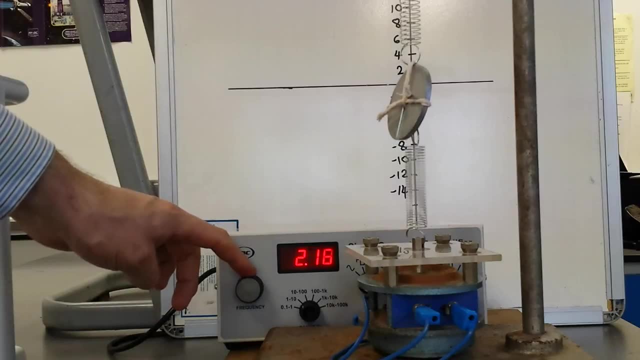 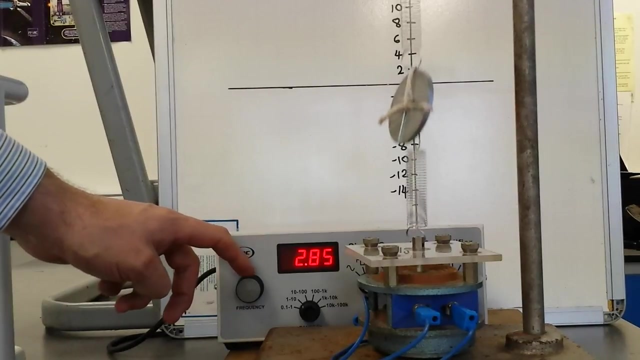 We're just looking for an overall effect. so two hertz. pretty much the same thing is happening. So let's go up a little bit more. there we go. two and a half seems to have died off. now there's not a lot happening. 2.7, 2.8, three hertz- interesting. 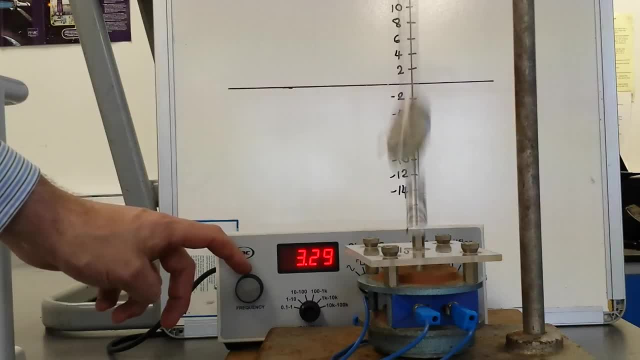 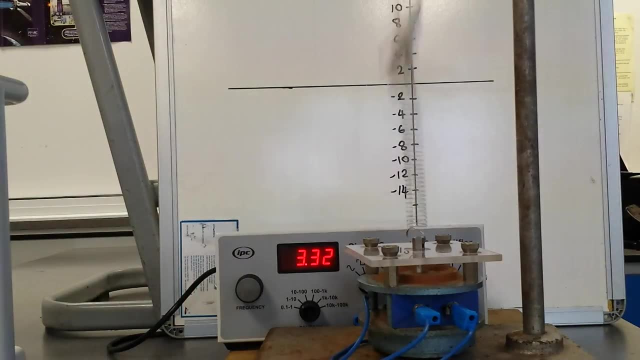 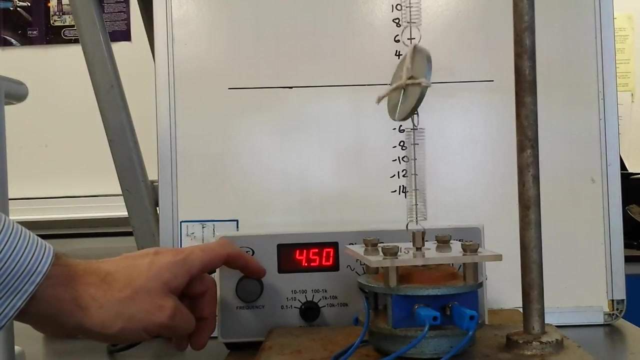 wow, 3.2, 3.3, crikey. the amplitude is massive, looking at least 14 centimeters. well, let's just go up a little bit more. 4, oh, oh dear, it's died off. 4.4, 5, 5, oh, it's gone. 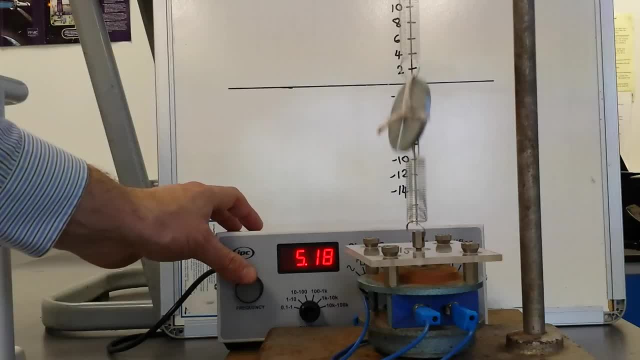 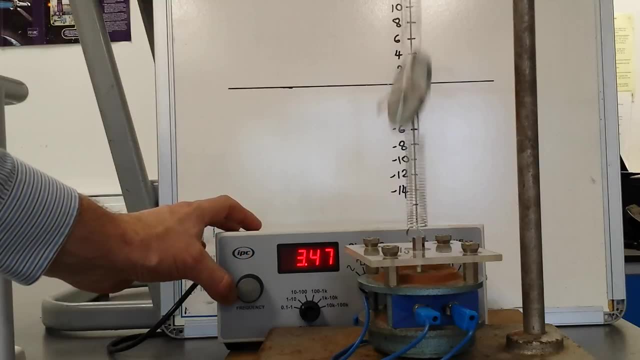 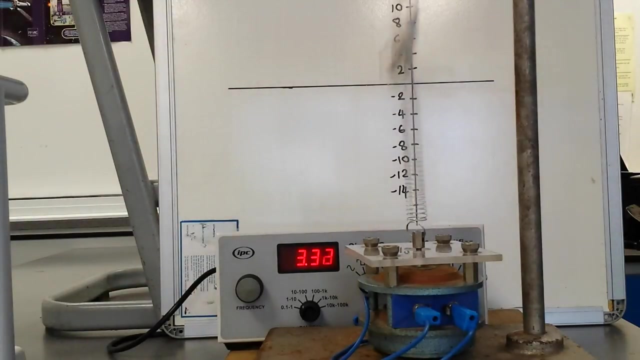 That effect is gone. let's go back now. I think it was roughly around the 3 point. yeah, 3.3, roughly looking about that. so we're clearly seeing a resonance effect. so what we're actually talking about is that when the frequency of the periodic 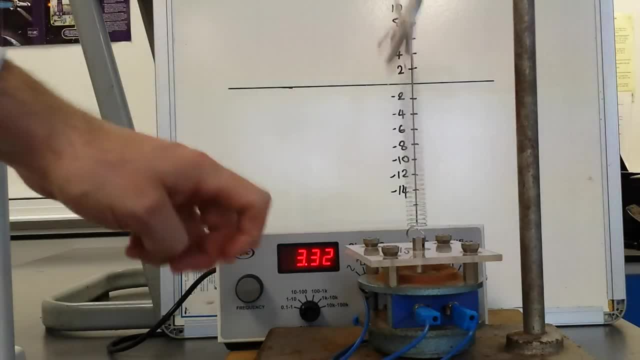 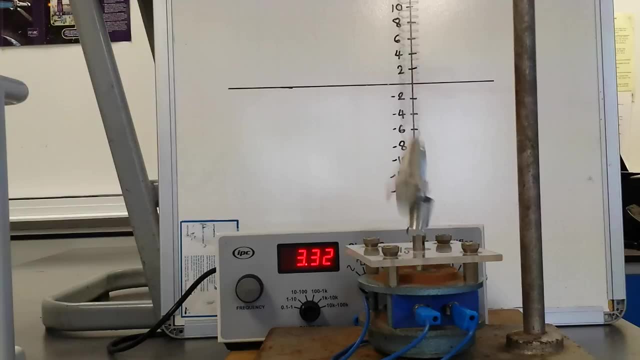 force applied. so the force that's applied here to the mass spring system equals what we call F naught, or the natural frequency. large amplitudes of oscillation occur providing the damping is line. now the periodic force needs to be in phase with the velocity, so force and velocity in phase of the oscillating. 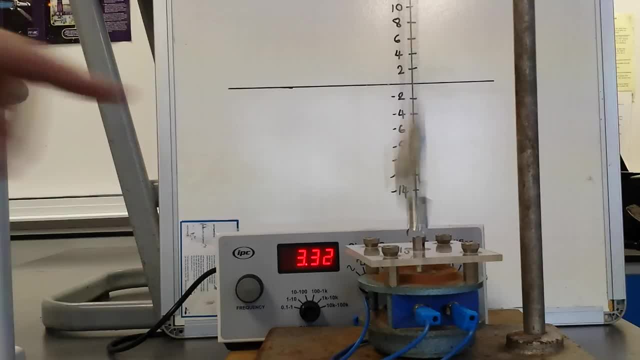 object: this occurs when the displacement- so the displacement here is pi- by 2 or 90 degrees, out of phase with the periodic force. now, as the applied frequency becomes increasingly larger than the natural frequency of the mass spring system, you saw clearly, didn't you, that the amplitude of the oscillations